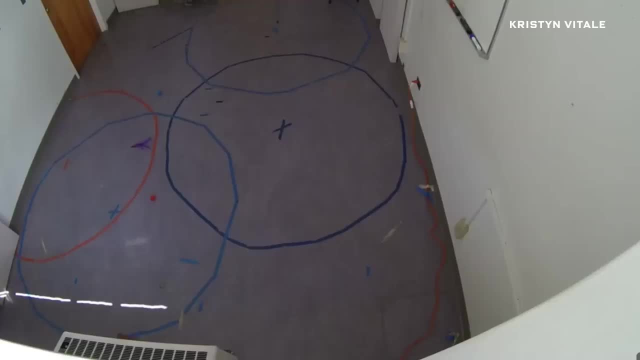 meows they produced basically, And then when the owner came back we looked at again the number of meows, so if those went down, And we found that when the owner was gone there was high rates of vocalizations, so high rates of separation distress, which then were relieved once that. 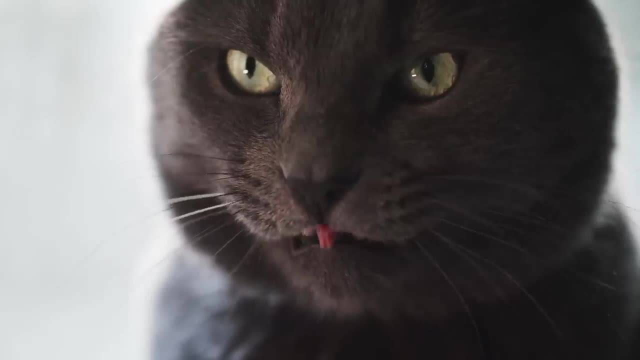 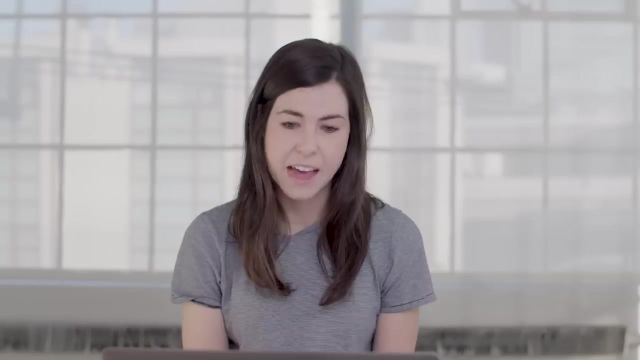 owner came back. There's definitely other behavioral measures, but we're looking at how they react to that return, The lip licking and the tail twitching, which are things we didn't actually measure in the study, but we just noted in the cats. And on those metrics, how do cats compare to dogs or even humans? 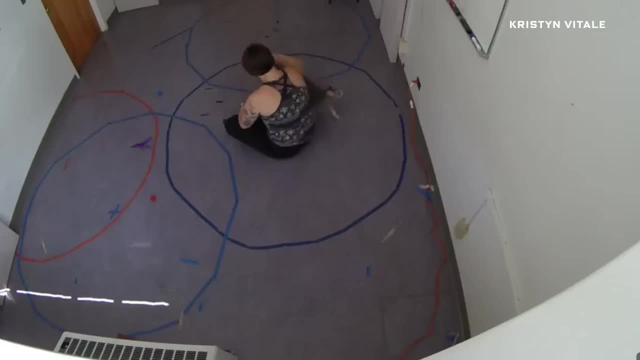 We see that the majority of cats react in a secure way, which means that when their owner comes back to that room, they go to their owner, they get attention and then they go back to exploring the new environment. And so there's this contact, exploration balance. But an insecure cat will. 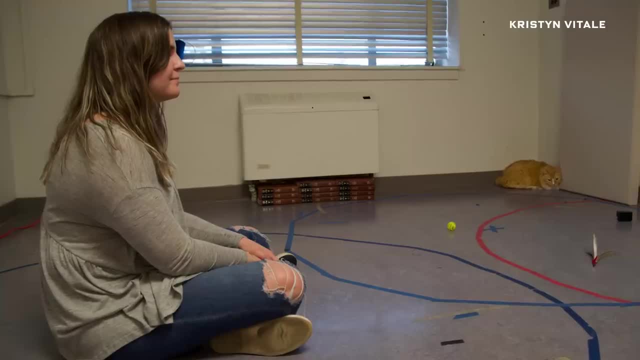 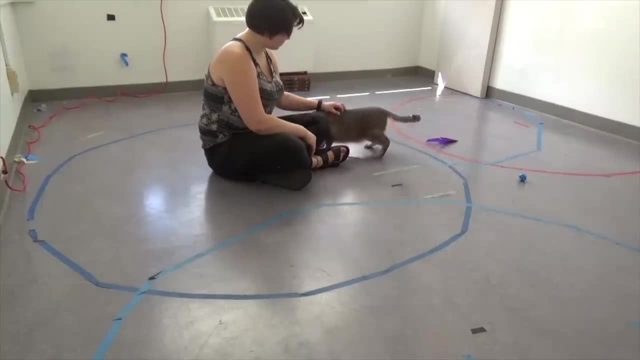 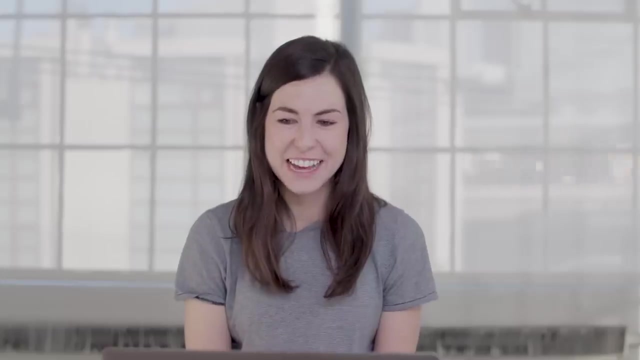 actually either excessively cling to their owner or excessively avoid them. The majority of both cats and kittens were securely attached- around 65%- And these are the exact same responses that we see in dogs and humans and at similar rates. That sounds like something a cat lover would say. 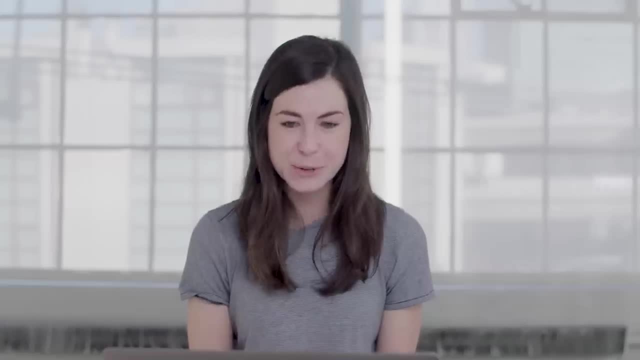 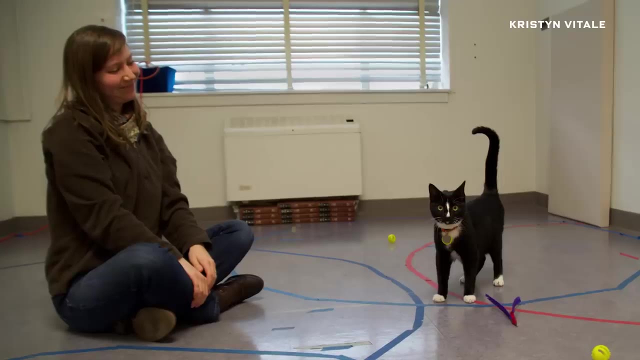 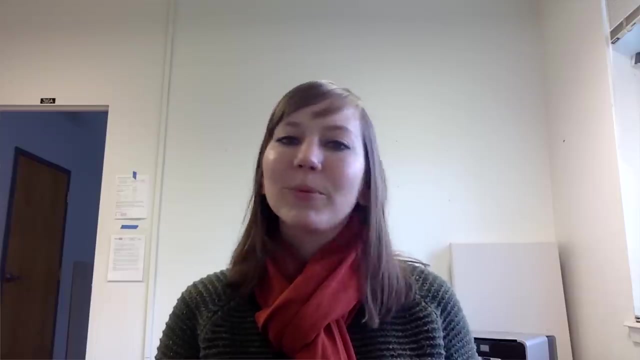 Hey, that's what we found. So when you were sourcing cats for this study, where did they come from? We recruited from the general public, So they came from our community. They came from Oregon State University students and employees, and word of mouth through different shelters, So just all over the place. Oh, I bet some of those people. were super happy to hear that their cats genuinely missed them when they were gone. Yes, there were a lot of people who were excited by this. for sure, The study was relatively small. You have sort of just over 100 cats running around your lab. 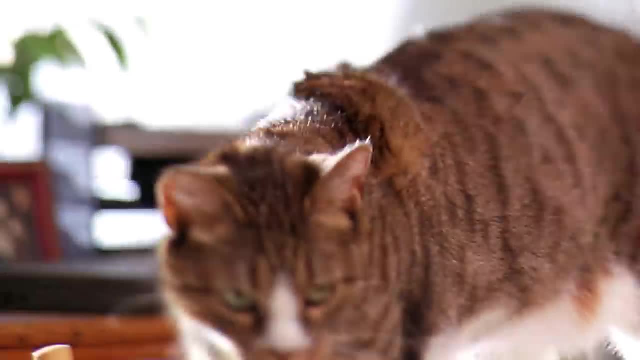 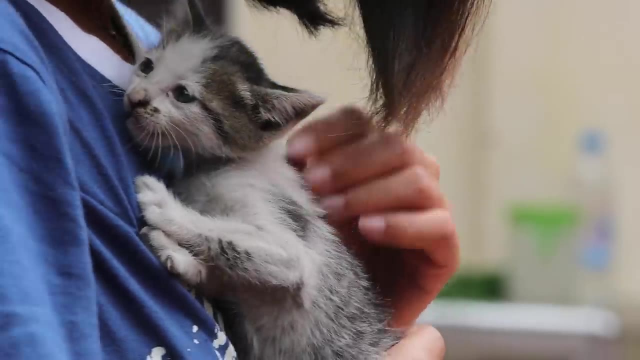 And for someone like me who's not a cat owner and has had a lot of aloof with cats, it makes me wonder, you know, is that atypical, Or am I just sort of not experiencing these kinds of attachment bonds because I've never had a cat myself? Actually, in a previous study, 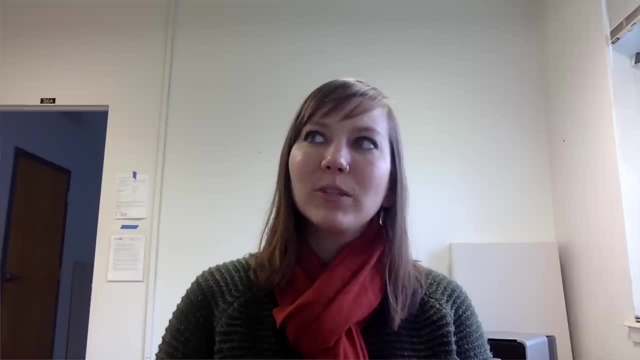 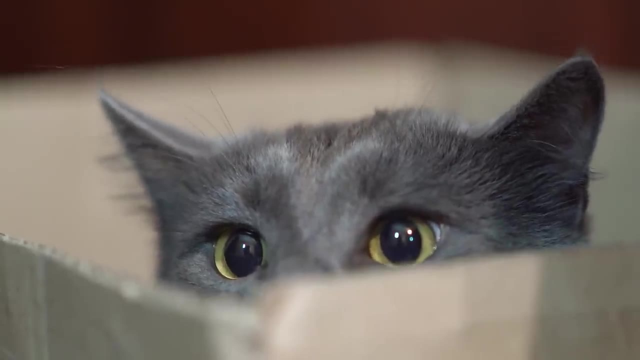 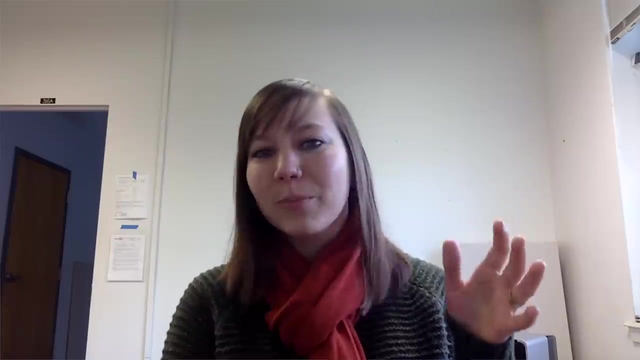 we looked at cat sociability And what we found was just a really great range in how social cats are. So we do see cats like you're describing that are really independent and maybe don't prefer social interaction. But then we see, you know, cats that kind of prefer it, cats that usually 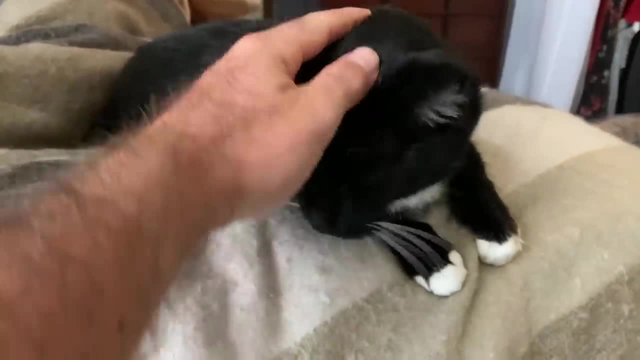 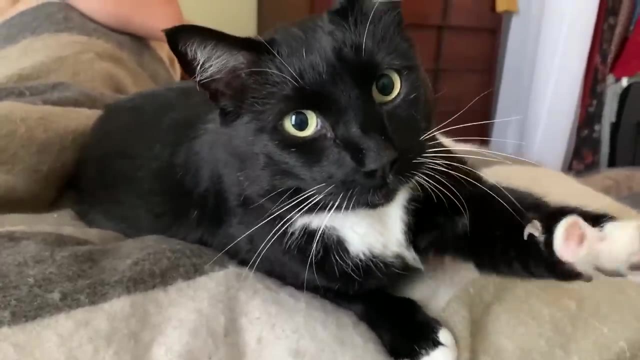 are really highly social. So we see everything in cats And I think this current research really indicates that even if your cat is fairly independent, they still seem to depend on you as a source of security. So, even though they might not be love bombing you all the time. 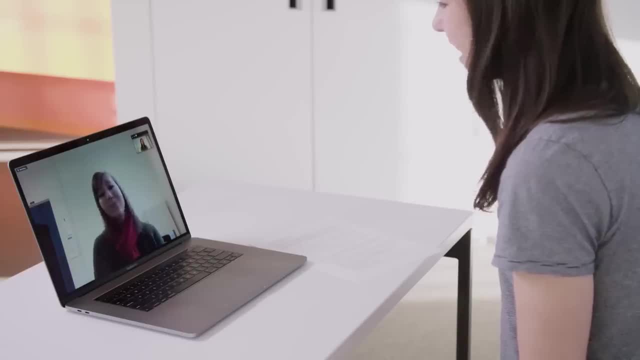 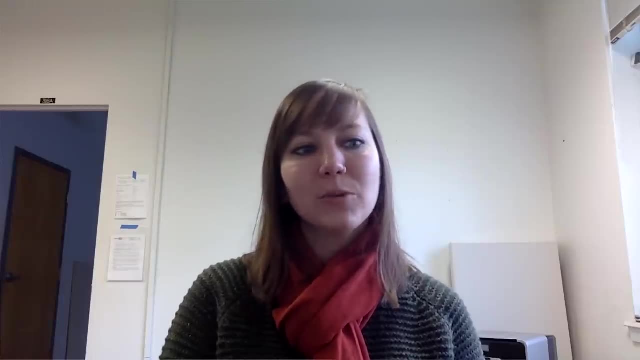 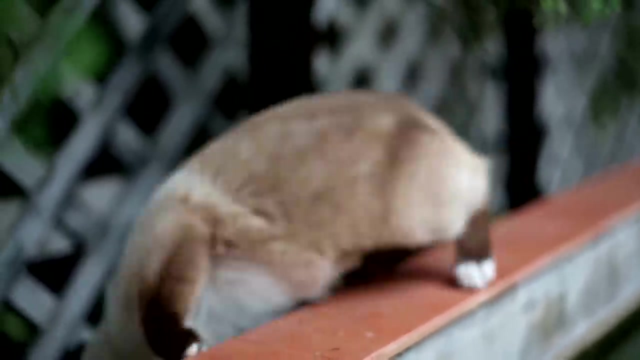 they're still viewing you as you know, that comforting factor. Then why are cats so mean? sometimes It's just like people, It's just like dogs. You know, you have some individuals who are more mean or more aggressive, but you have plenty of individuals who aren't, And I do think some of it comes down. 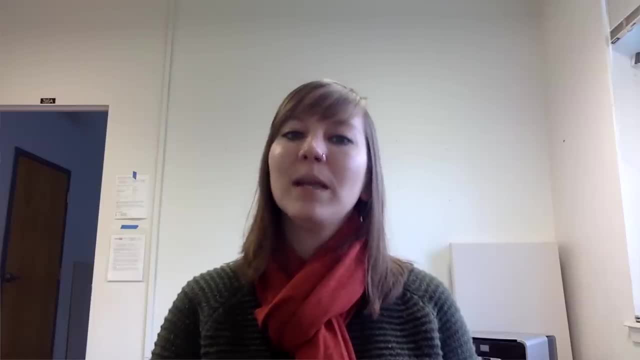 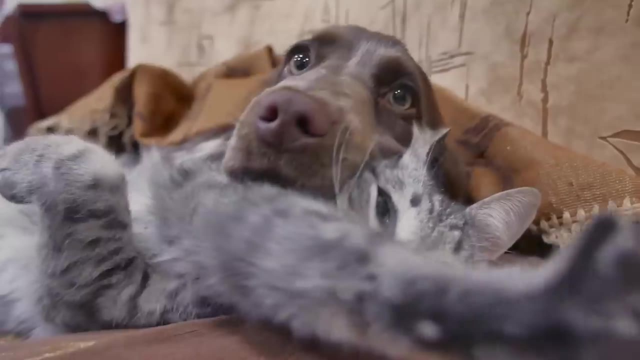 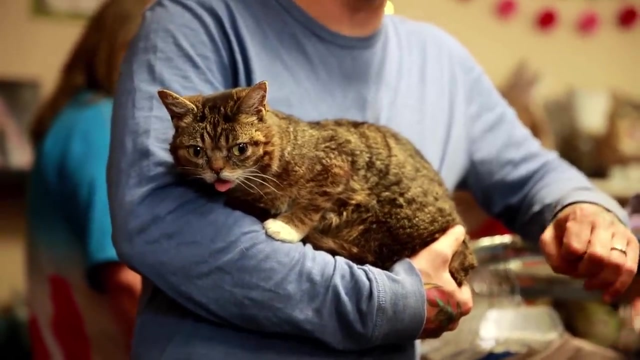 to people, maybe misreading cat body signals or maybe not knowing how to interact as well. Cats don't have as many facial muscles as dogs do, So I think that sometimes they look maybe more upset than they may seem, especially if we're comparing them to dogs, you know. 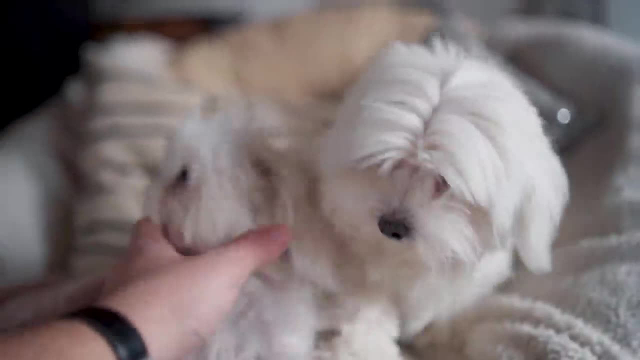 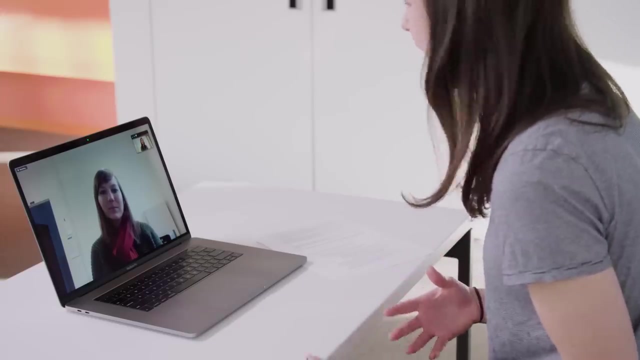 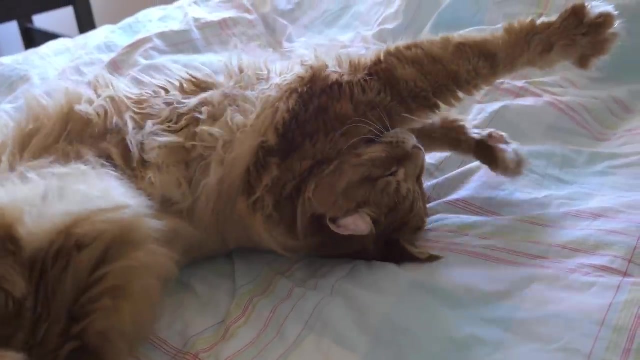 have their mouths open and their tongues out. I think it's easier for people to kind of read that body language than with cats. So what do we actually know about what's going on in a cat or a dog or any other animal's head when we're studying them in this way? Like can we say definitively that a cat is feeling one? 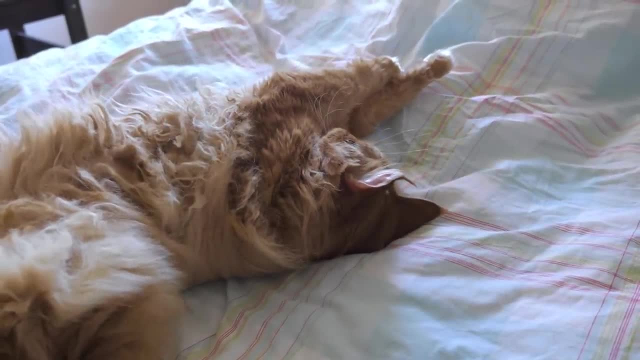 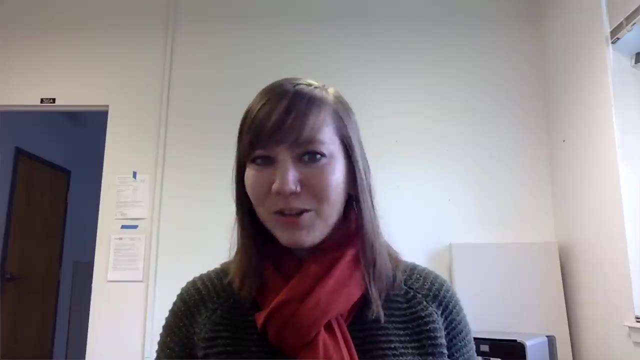 thing or another, Or are we sort of just making our best guesses based on previous studies in humans? You don't want to assume too much And we don't really know what love in a non-human fashion means. You don't want to anthropomorphize or attribute human traits to the animal. 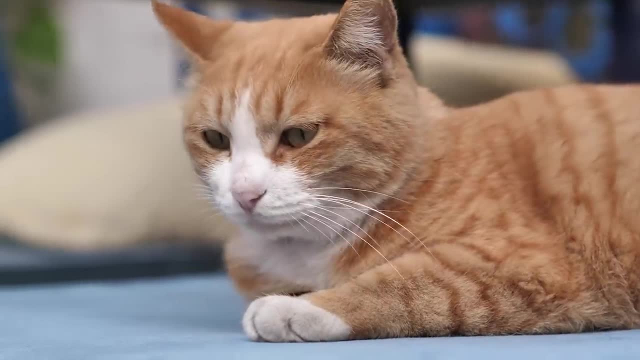 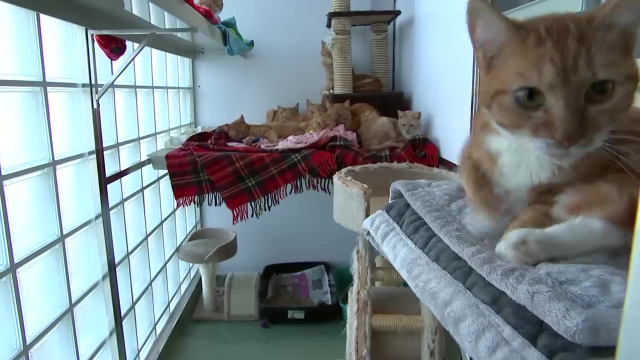 You always want to be careful of that. So it's really through reading their body language that we can say if they're behaving in a secure or insecure way, But we can't really say what that means for them- that if they behave in a secure way, that means they love their owner. It might 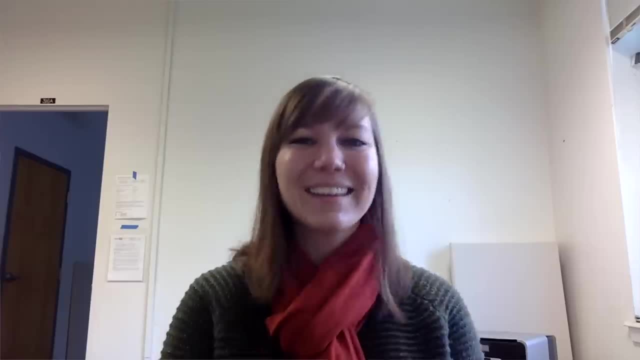 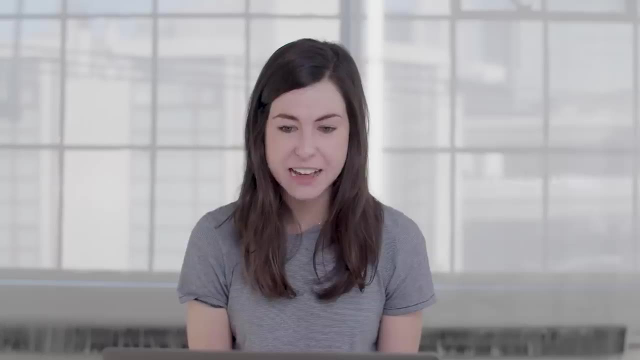 mean that, but we can't really say that because we can't ask the cat. So, in light of what you've sort of discovered recently, what are some future research questions that we still have around cats and the way they relate to humans? So in our current study we're looking at how cats react to humans. 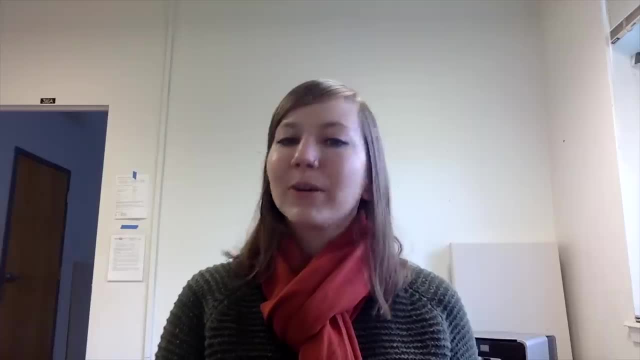 So in our current study we're looking at how cats react to humans. So in our current study we're looking at how cats react to humans. So in our current study we only looked at the behavior towards the owner. Other attachment studies also look at the cat's behavior towards a stranger, an unfamiliar person. So that's.